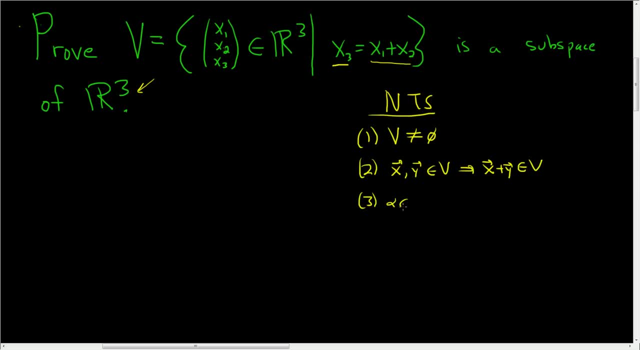 And lastly, we have to show that if we have, say, a scalar alpha in our field, which is the set of real numbers, and another vector in V, that the scalar product, so alpha X, is also inside V. So we have to show it's closed under vector addition and this here is saying it's closed under scalar multiplication. 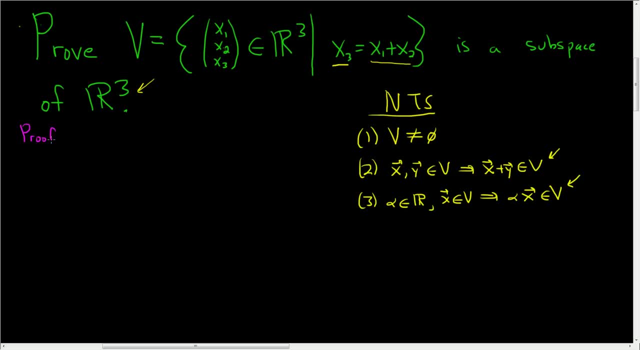 Let's go ahead and prove this. It's a pretty easy proof, So proof. So we'll start by showing condition one. We have to show it's not empty. We'll note that zero is equal to zero plus zero, Right, so zero is equal to zero plus zero. So this means that the vector zero, zero, zero is in V. 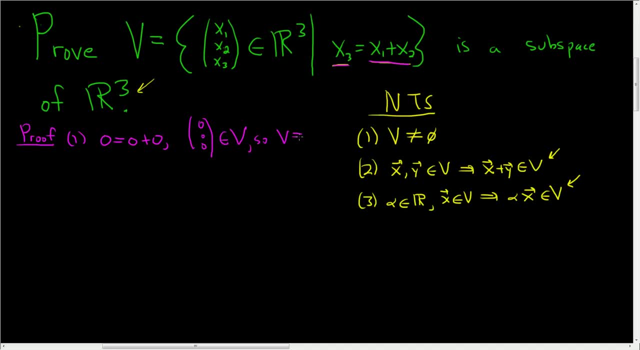 So we have to show it's closed under vector addition. So it does contain the zero vector, so it is in fact non-empty. So condition one is done, Pretty easy. Two: we have to take two vectors in V and show that their sum is also in V. 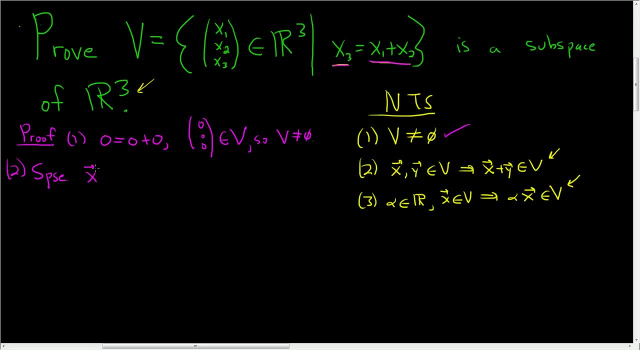 So suppose that we have two vectors which live inside V, Then that means we can write these vectors as follows: That means that the first vector, X, is X1, X2, X3.. And the other vector, let's call it Y1, Y2, Y3, for sum. 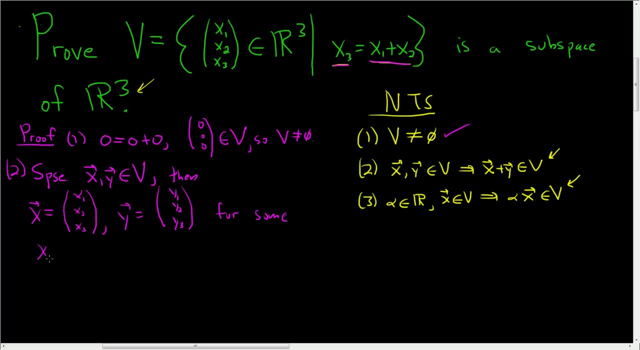 And then we know that all of these little components- X1, X2, X3, these are all real numbers: Y1, Y2, Y3.. These guys are all in the set of real numbers And, moreover, we know something else: This is a special set, right. 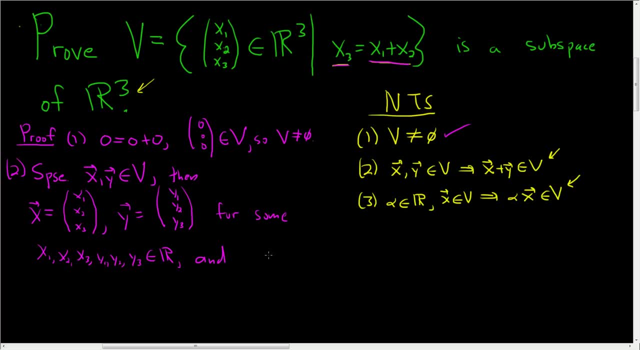 If you're in this set. If you're in this set, your third component is the sum of the first two. So, and we know that X3 is equal to X1 plus X2, and Y3 is equal to Y1 plus Y2.. 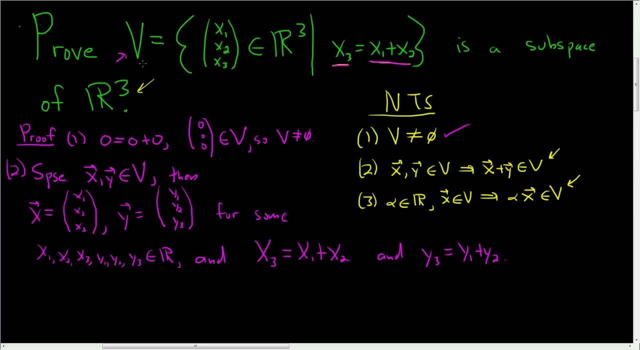 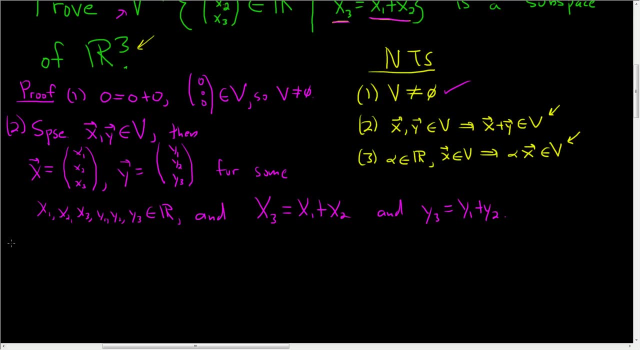 So we know that's what it means for a vector to be in V. It means the third component is the sum of the first two. Now we have to show that the sum is in this set. So note, let's look at what the sum looks like. 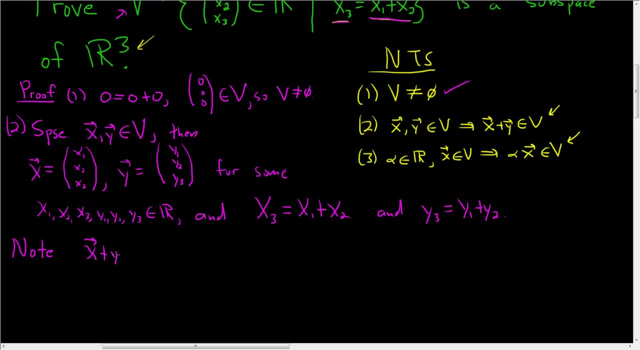 If you take X, If you take vector X and add it to the vector Y, well, the addition is the normal component-wise addition. So you just add the corresponding components, So X1 plus Y1,, X2 plus Y2, and X3 plus Y3. 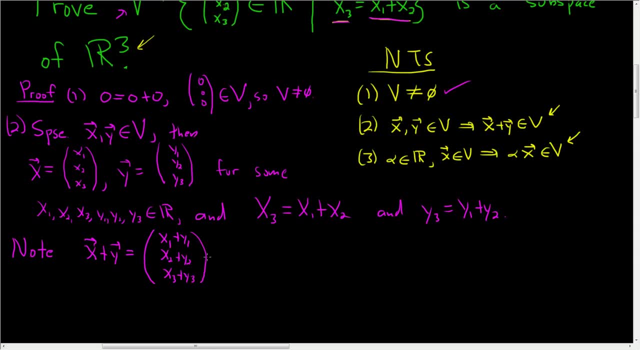 So that's what the sum of the vectors looks like And we have to show that this is in V. So we have to show that the third component, So, and The third component- X3 plus Y3, we have to show it's the sum of the first two. 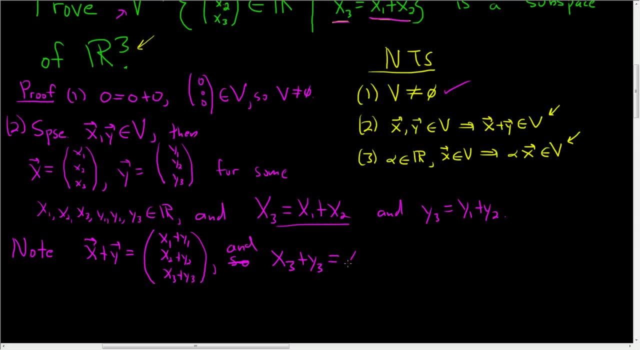 Well, X3 is right. here It's X1 plus X2.. And Y3 is right. here It's Y1 plus Y2.. And I'm being a little abusive here, You should have parentheses, but these are real numbers. 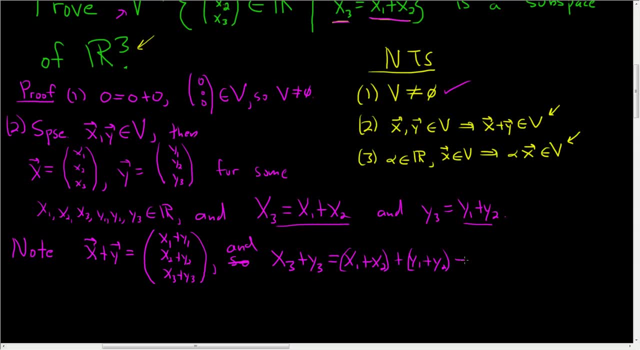 So addition is associative and, moreover, it's commutative. So we can write this as X sub 1 plus Y sub 1 plus X sub 2 plus Y sub 2.. So we've shown that the third entry, the third component of our vector, 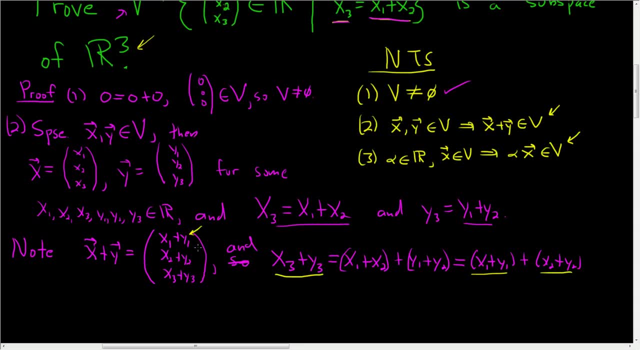 is the sum of the first two. right, The first two. That's precisely what it means for the vector X plus Y to be in V. So X plus Y is in V. So this shows that V is closed under vector addition. The third step is to show it's closed under scalar multiplication. 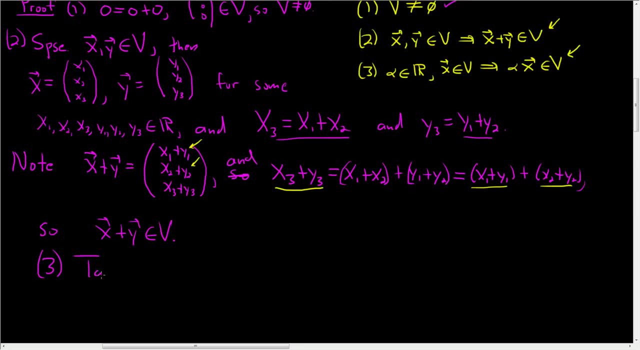 Again, pretty easy. So take any vector in V and some scalar alpha in the field of real numbers. Then we know that X is equal to the vector whose components are X1, X2, X3. for sum X1, X2, X3. 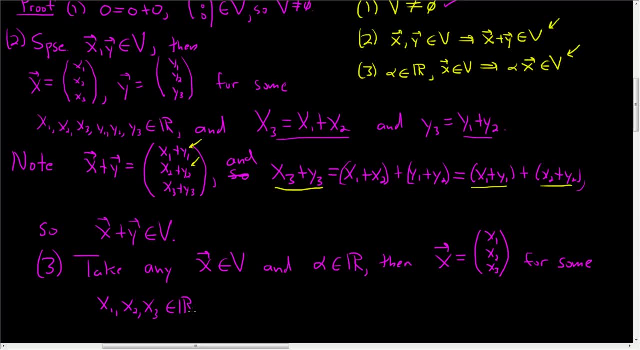 in the field of real numbers, And we know that the third component is the sum of the first two. So X3 is equal to X1 plus X2.. So then we have to look at the vector alpha times, the vector X, The vector alpha X. 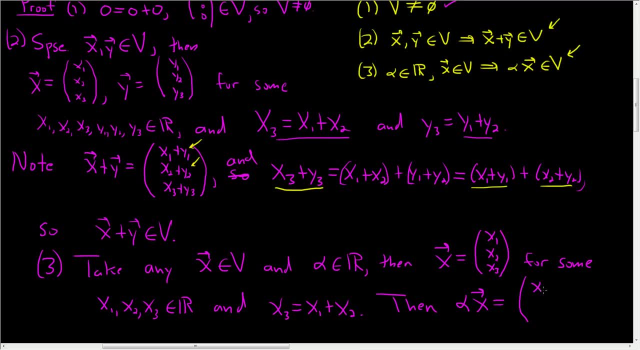 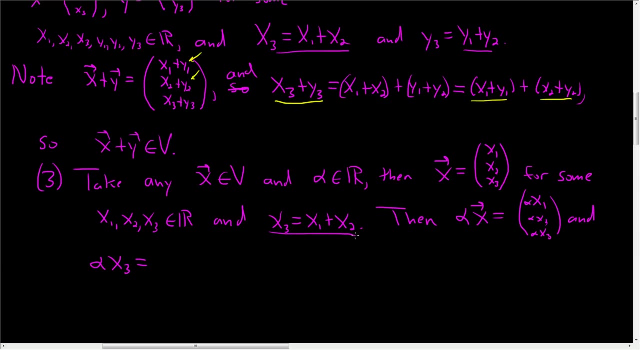 So this is equal to X sub 1, alpha X sub 1, alpha X sub 2, alpha X sub 3.. And Well, what is the third component? Alpha X sub 3.. Well, using this equation, that's alpha times X sub 1 plus X sub 2..